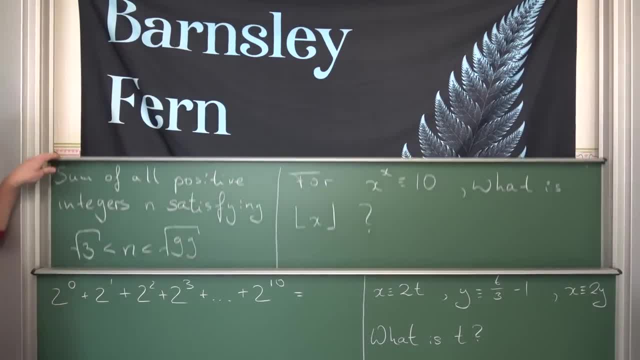 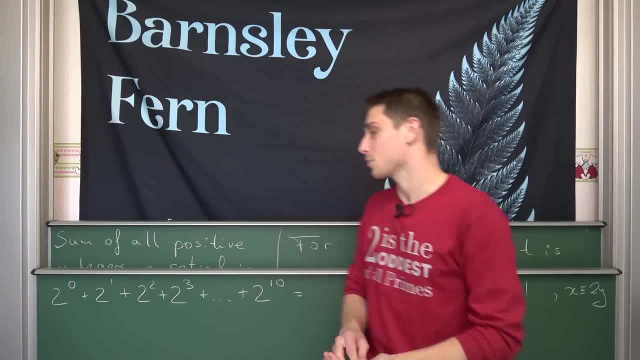 for yourself. They are just cute and very small and easy to solve. but I thought I would end this on a very chill note here on the Advent Calendar And now we are going to dive right in. So the first problem involves a summation of powers of 2. 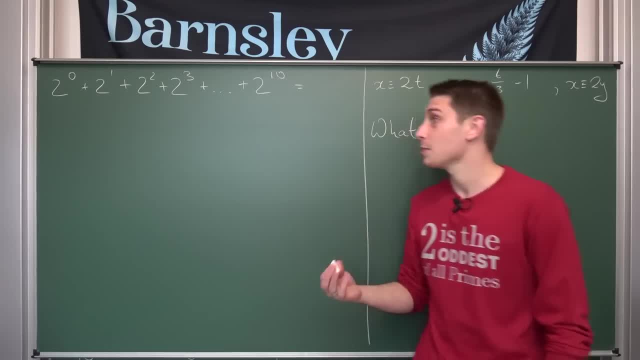 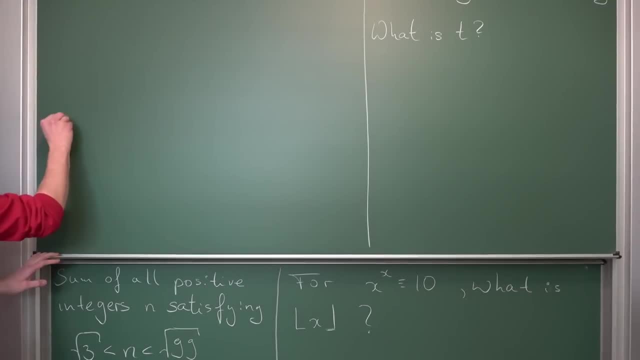 and the way to go here is, I think, by the geometric series. that's the easiest thing you could possibly do. Let us remember what the geometric series looks like. So if we have some kind of x to the 0th power plus x to the 1st power plus, 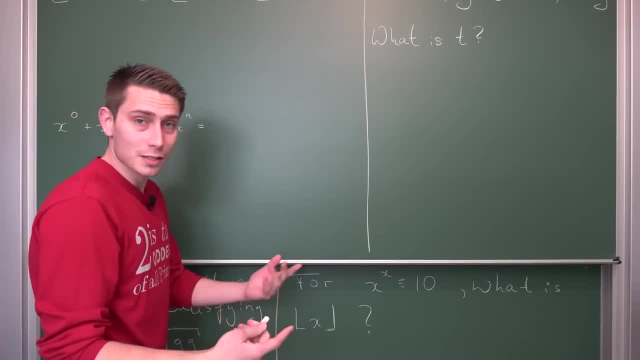 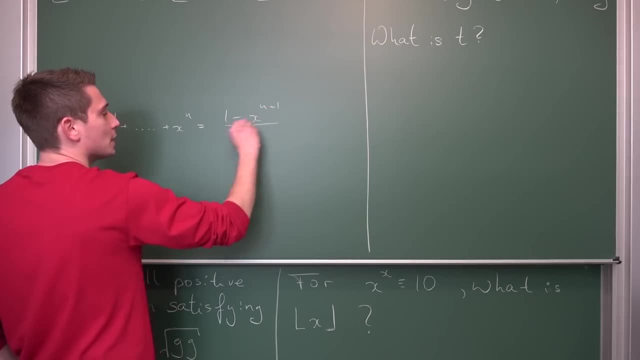 up until x to the nth power. we can actually rewrite this, so maybe link in the description to the corresponding video as being nothing but 1 minus x to the n plus 1th power divided by 1 minus x. So now we just need to identify. 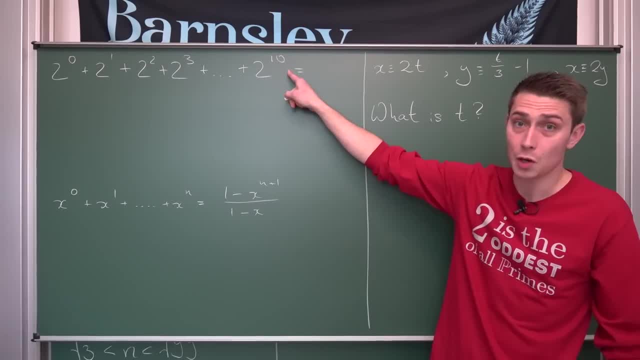 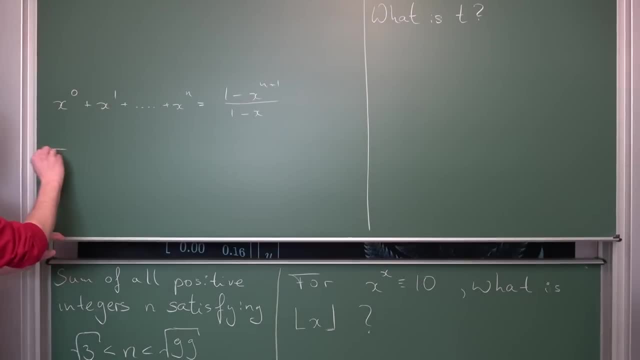 what our n actually is, so the highest power of 2, which is 10.. Okay, n is equal to 10. and also what the base is. Well, the base, obviously, is 2, meaning, in our case, for n being equal to 10 and x being equal to 2. 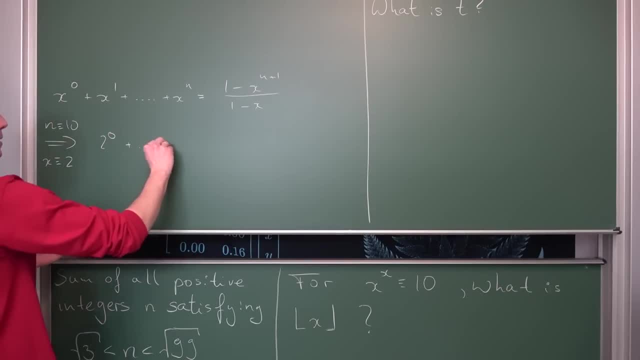 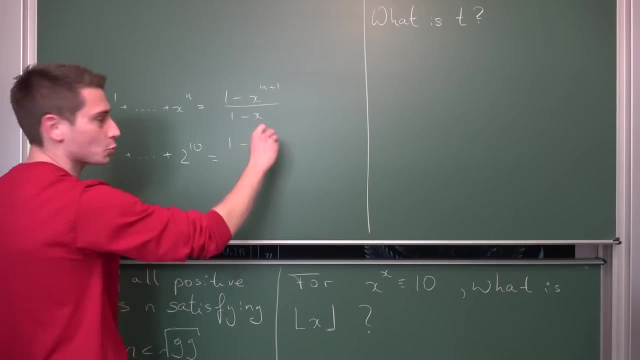 we are going to get that 2 to the 0th power plus up until 2 to the 10th power is going to result in: okay, we are going to get 1 minus 2 to the 10. plus 1 is nothing but 11. 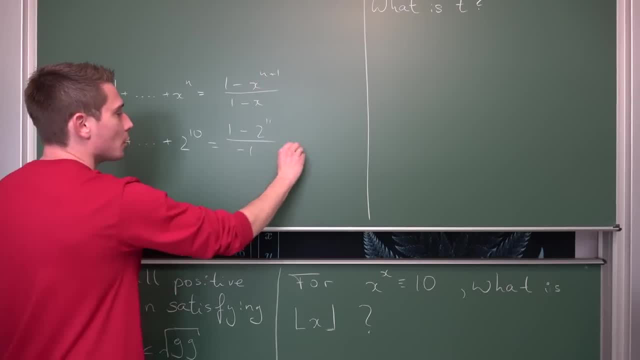 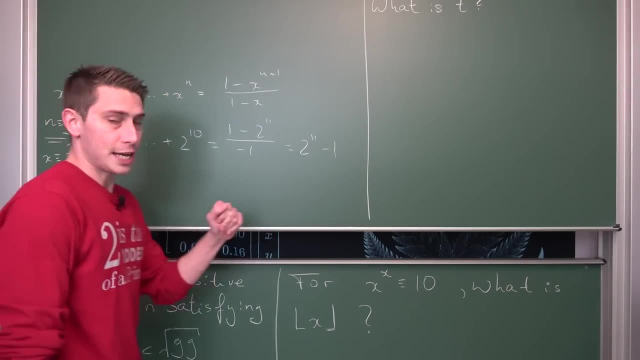 divided by okay, 1 minus 2 is negative 1, which is going to result in distributing the negative sign into here in 2 to the 11th power minus 1.. I mean 2 to the 10th power is 1024, so 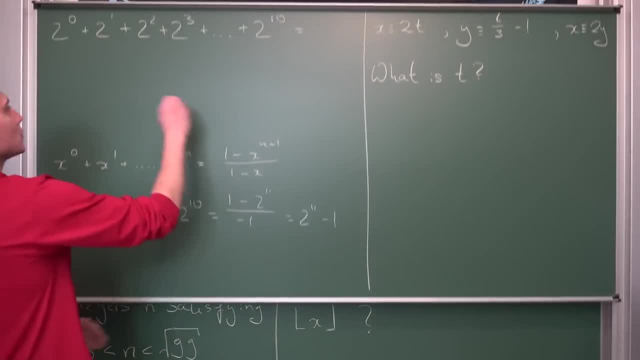 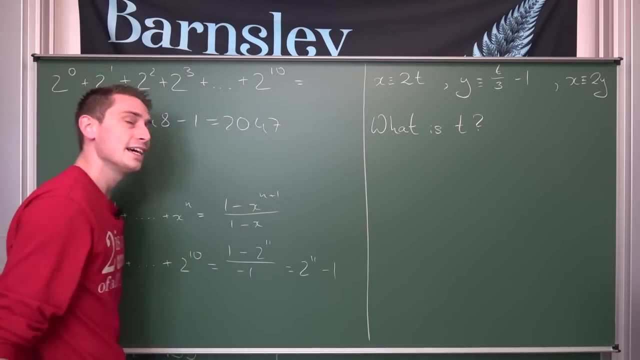 this times, 2 results in 2 to the 11th power, resulting overall in 2048 minus 1, which is nothing but 2047, and hence we are done. Quite easy, right, But cute. I like puzzles like those. Now next up is 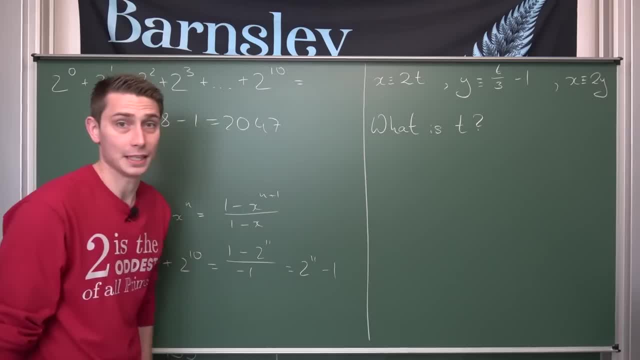 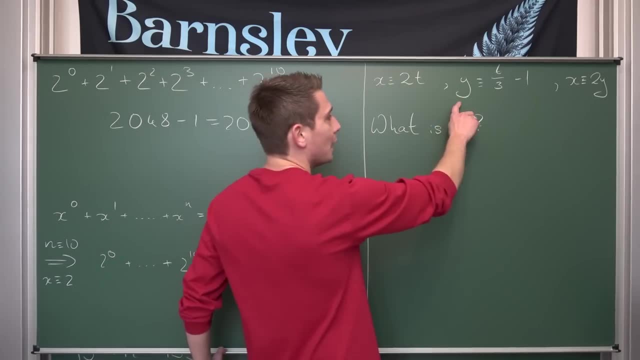 what is the value of t with those conditions given up here, and it's actually really easy to find out once again. So at first we know what x is. It's equal to 2 times t, and now we are going to multiply y by 2 because we want to. 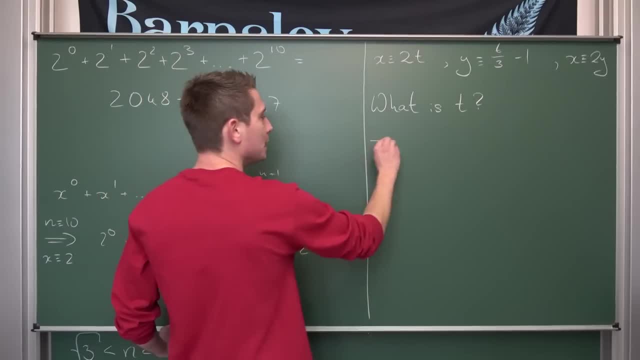 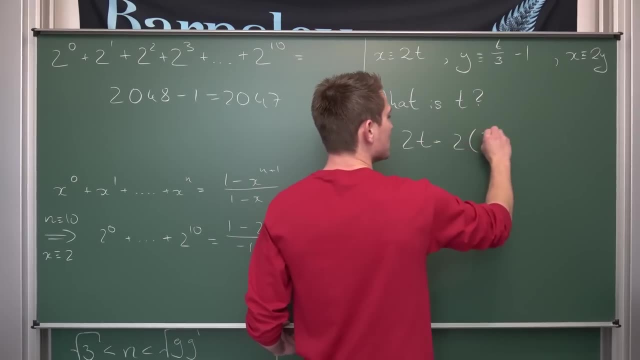 find out what happens if x is equal to 2y, Meaning overall, since x is nothing but 2t. this is hence equal to 2 times this quantity right here, So 2 times t over 3 minus 1.. I mean 2. 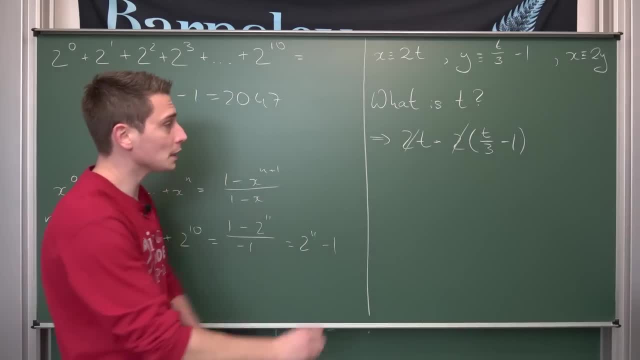 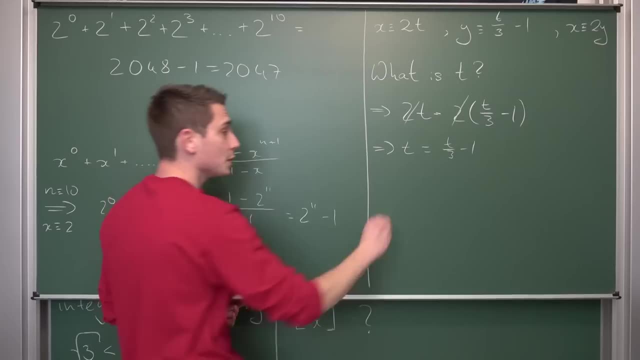 is not equal to 0. we can just divide both sides by it, leaving us overall with t being hence nothing but t over 3 minus 1.. We can subtract t over 3 on both sides t thirds, so t minus t over 3. 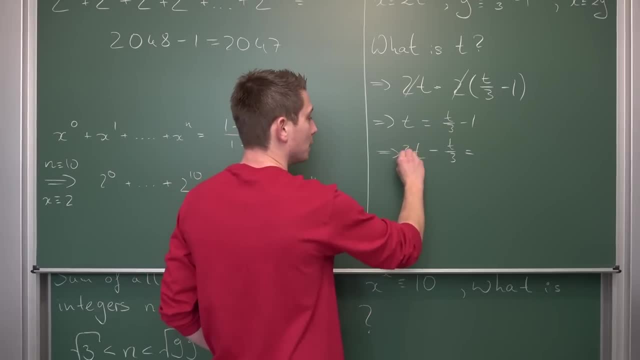 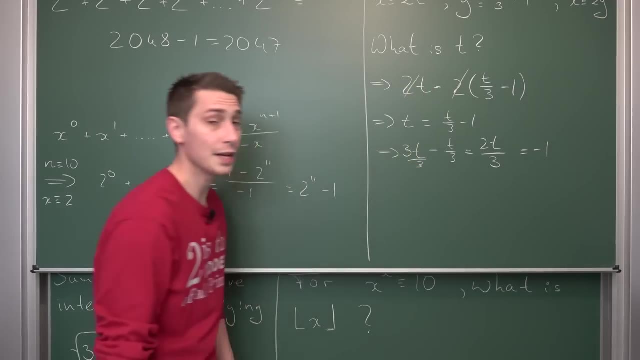 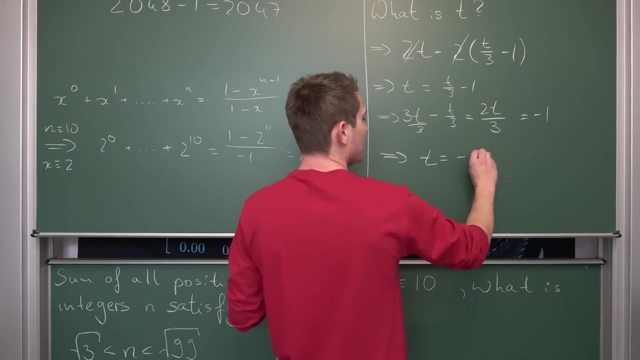 hence nothing but okay. expanding this t by 3 over 3 results overall in 2t divided by 3, being hence nothing but negative. 1 and now multiplying both sides by the reciprocal of 2 thirds is going to result overall in t being nothing but negative. 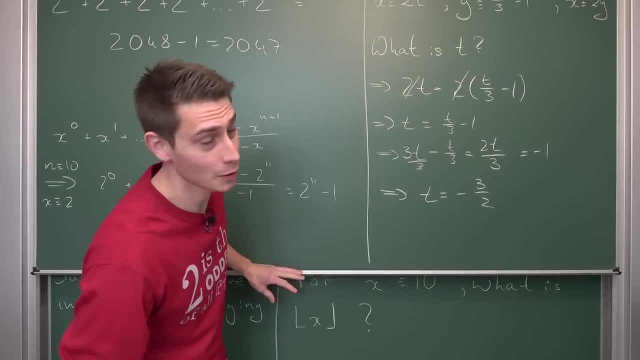 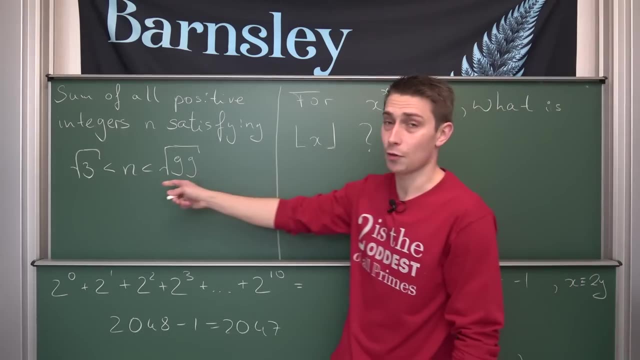 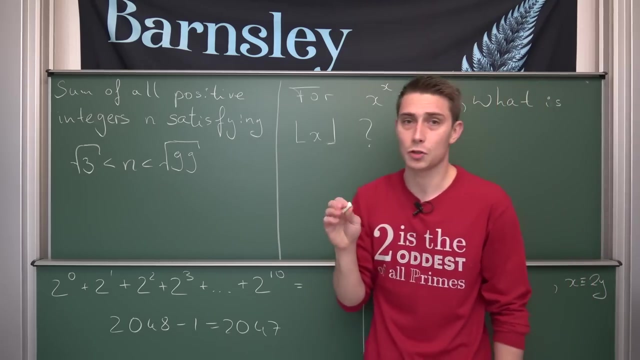 3 over 2, and hence we are done. You probably got that right too. Now next up: what is the sum of all positive integers n satisfying square root of 3 being less than n being less than square root of 99.. So at first, we are going to do some. 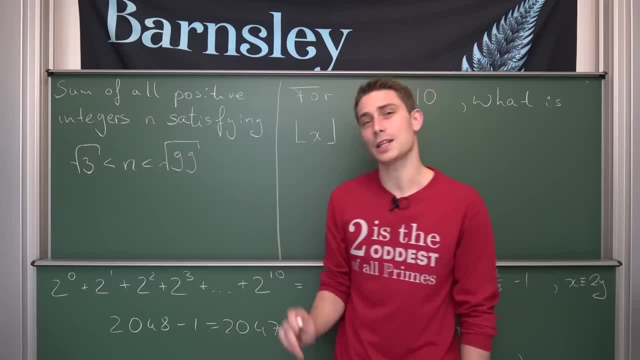 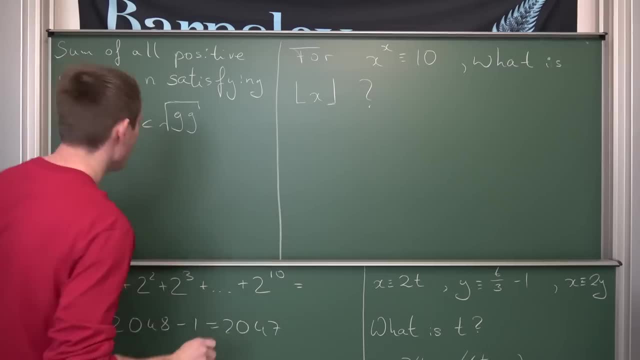 argumentations. here We are going to see how our square roots are actually bounded in this problem. and n is a positive integer, meaning we need to round stuff up and down in the process. I mean, if we take a look 3, what are the nearest perfect squares? 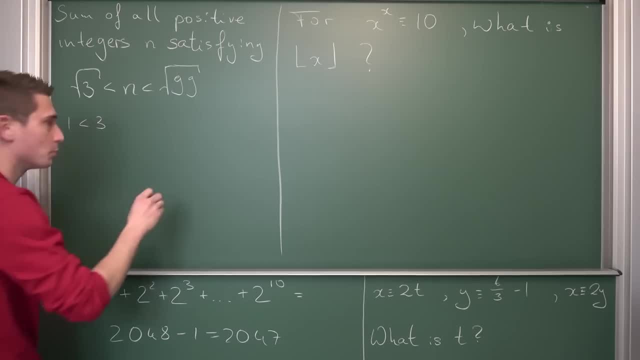 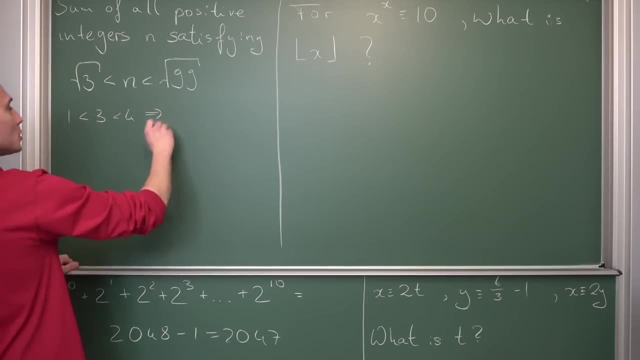 I mean 3 is greater than 1. obviously, 1 is a perfect square and 3 is less than 4.. 4 is the next nearest perfect square. meaning taking the square root on each and every term right here is going to result in: 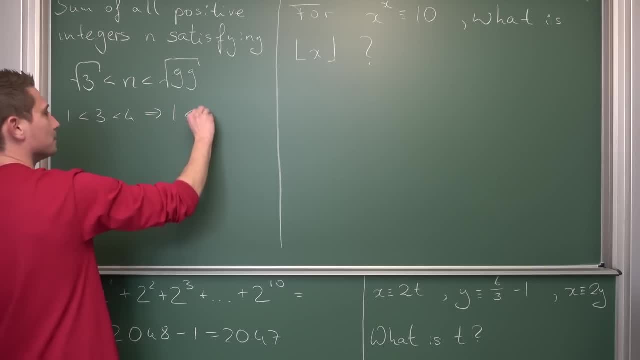 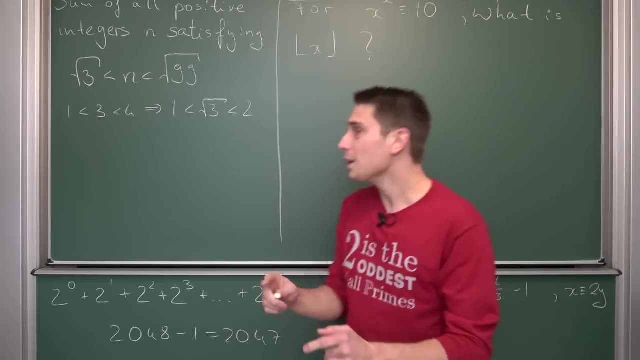 square root of 1 is nothing but 1, being less than square root of 3, and this is less than okay. square root of 4 is nothing but 2, meaning square root of 3 is bounded between 1 and 2 somewhere, which does. 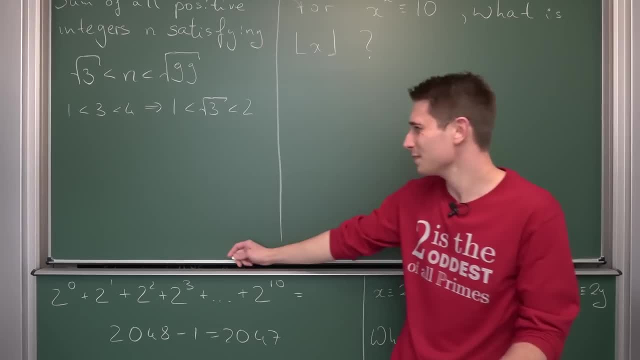 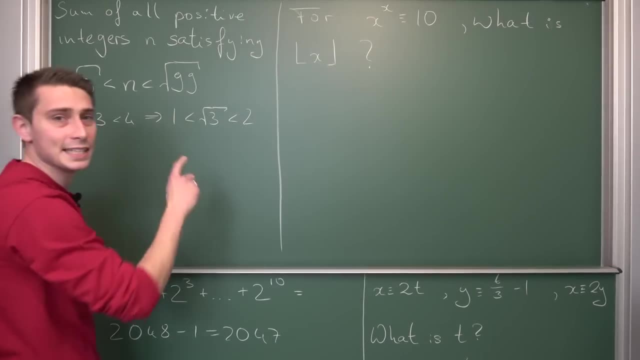 make sense. Square root of 3 is something like 1.7, I think. something like this. it's more than square root of 2. yeah, 1.7, something like this. and we are going to go through the same process. what are the nearest perfect squares to? 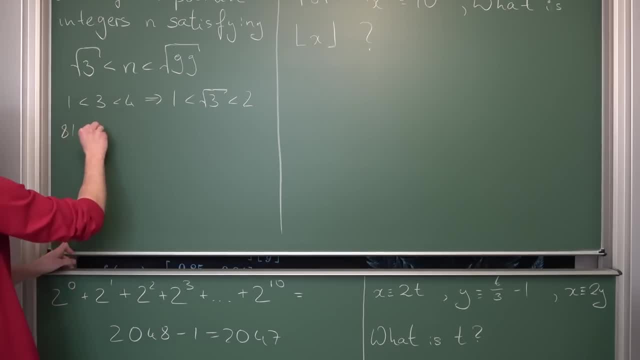 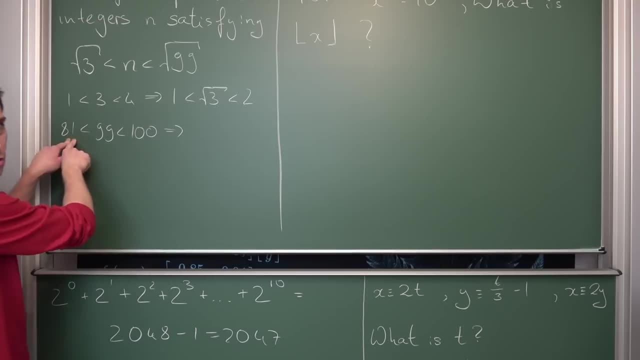 99, I mean 81 is 9 squared, so 99 is greater than 81 and the nearest perfect square to that is 100. meaning taking the square roots, okay square root of 81 is going to result in 9 being less than okay square root of 99, which is: 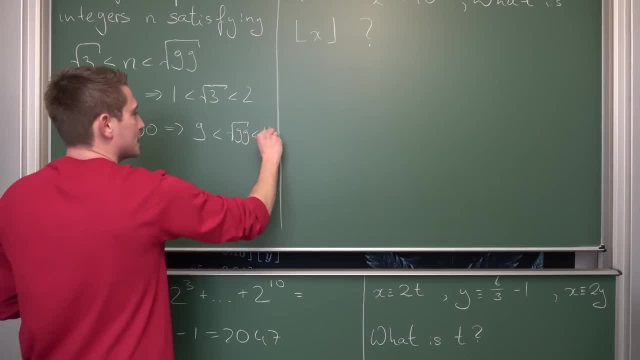 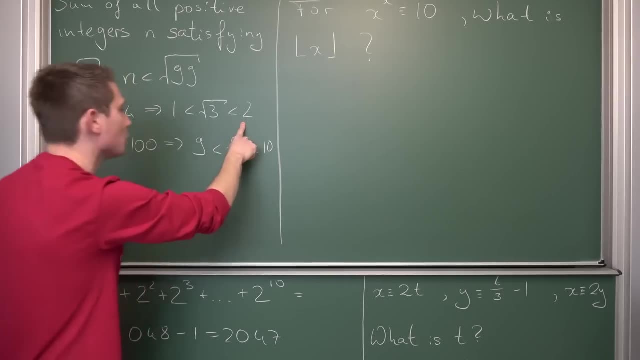 what we are striving for, and this is less than square root of 100 is 10, meaning overall n is thus bounded between: okay, n can be equal to 2, because n is strictly greater than square root of 3, meaning it could also be 2. so 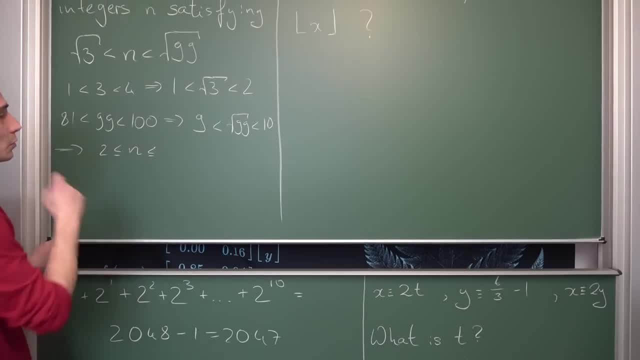 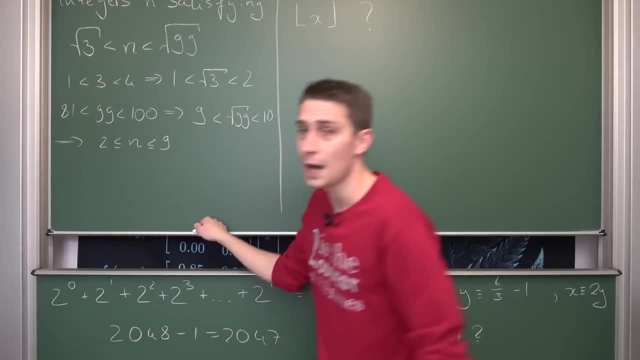 n is greater or equal to 2, which is less or equal to? I mean it can be 10, because 10 is already greater than square root of 99, but it could possibly be 9, meaning finding the sums of all the numbers that n could possibly take. 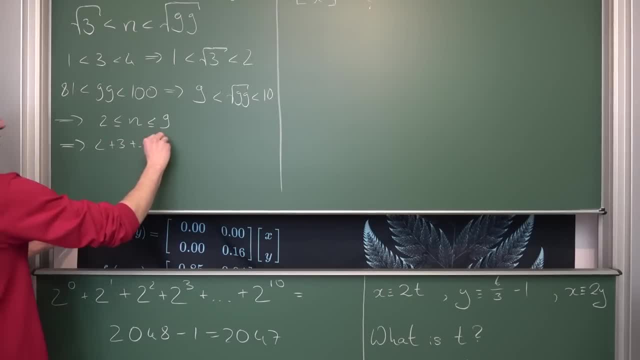 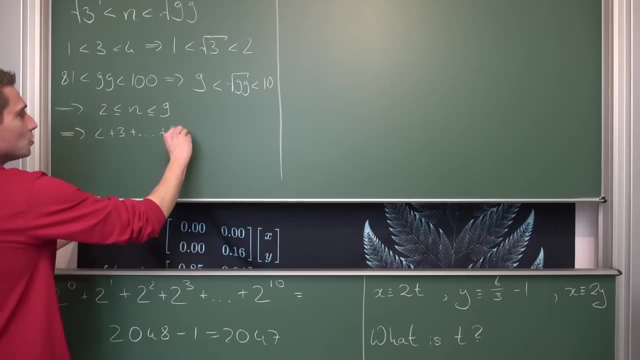 is going to result in 2 plus 3 plus up until 9, and yeah, you could just simply calculate this, or we are going to make use of little gauss. meaning what we are going to do is we are going to add a 1 and subtract it, meaning this part, right. 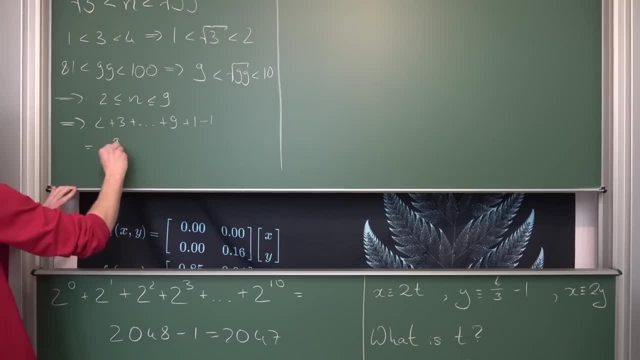 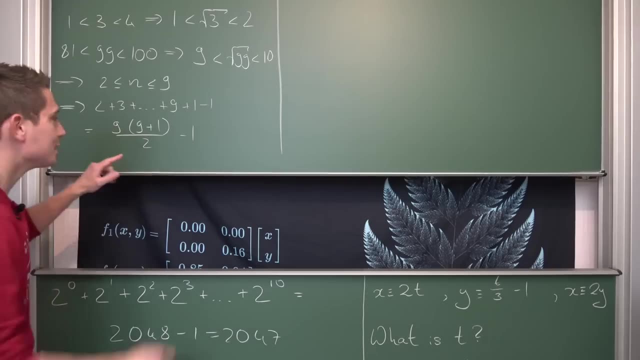 here is just going to be little gauss from 1 to 9, leaving us in 9 times 9 plus 1 divided by 2 minus 1. so 9 plus 1 is nothing but 10. 9 times 10 is 90. divided by 2 is: 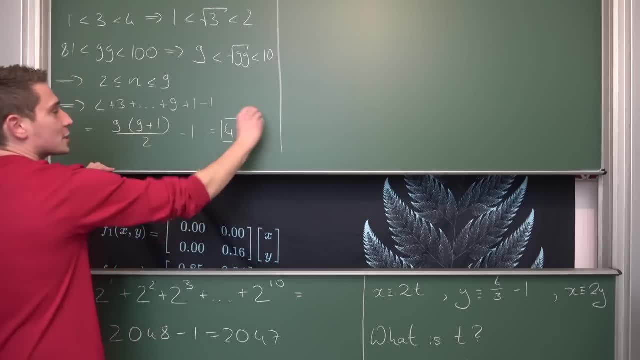 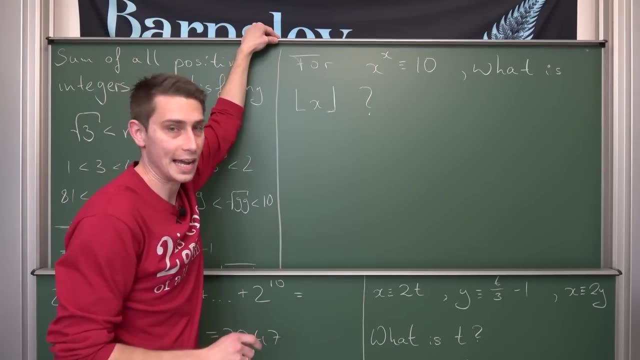 45 minus 1 is equal to 44, and hence we are done. now the last problem: for x to the x, power being equal to 10, what is the floor of x? floor of x meaning? it is like a rounding down function. so if you were to have, for example, 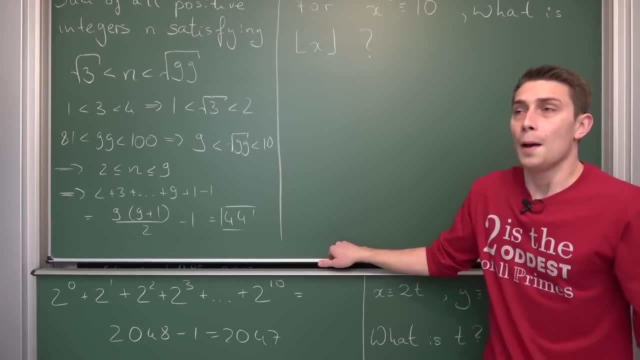 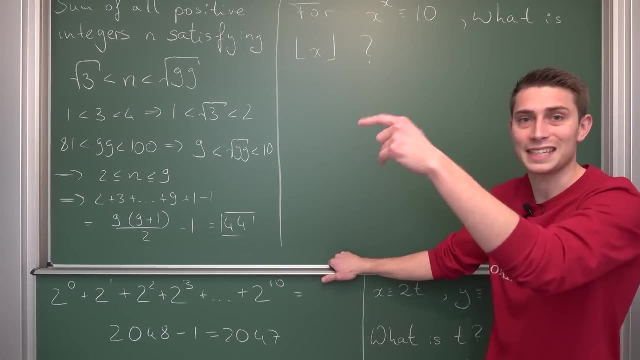 2.5, the floor of that is going to result in 2. but if you were to have- yeah, I mean you are always going to round down- if you have the floor of 2.99, it is going to be 2 yet again. so 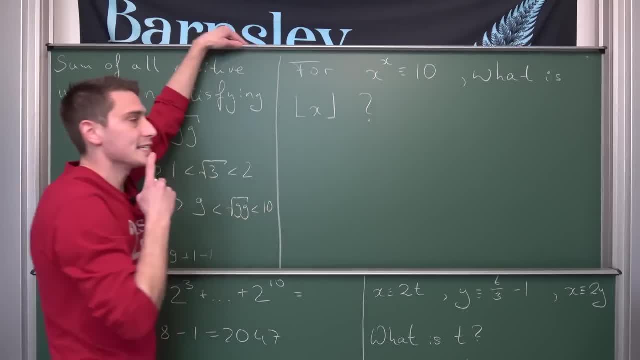 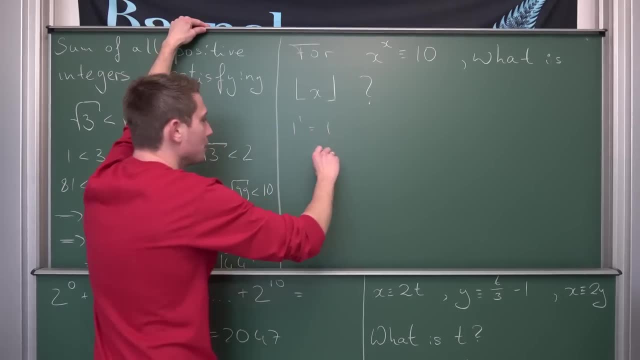 let us go through the process here. I mean x to the x. power is equal to 10, so let us bound x to the x power in some way. again, I mean 1 to the 1th. power is nothing but 1. now, what about the next? 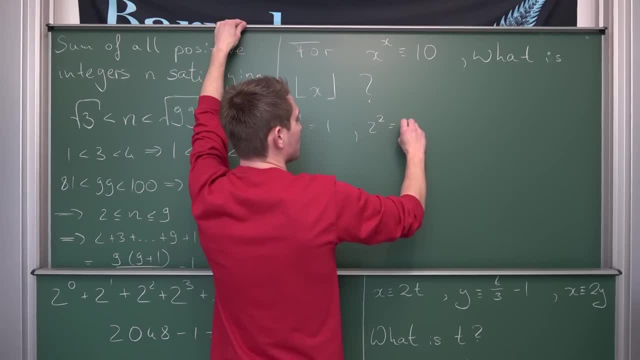 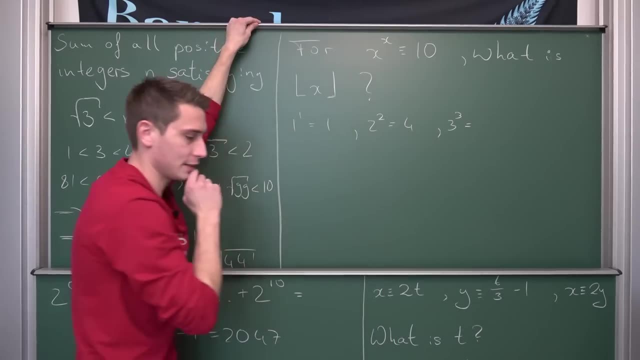 x to the x power. this is 2 squared, hence nothing but 4. ok, this is less than 10, and what else do we have? I mean we have 3 to the 3rd power. ok, 3 squared is 9 times 3 is going to give us 27. 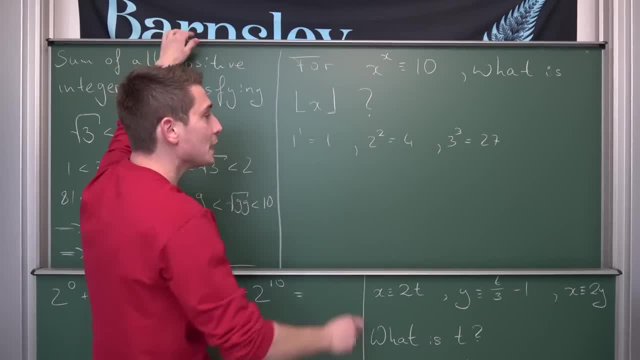 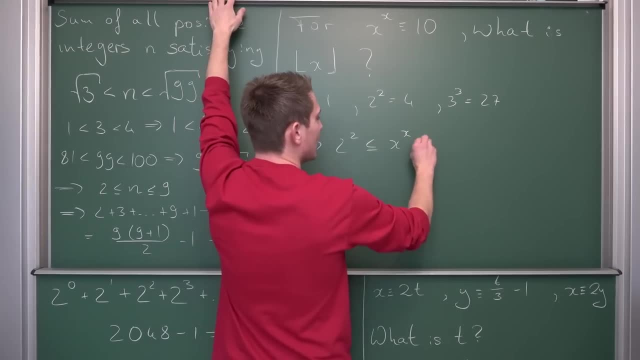 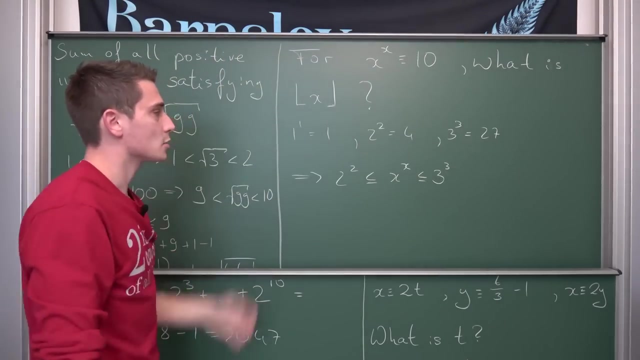 meaning overall, our x to the x power, which is equal to 10, is somehow bounded between 1 to squared ok and our 3 cubed. it is bounded like that. I mean x to the x power must be equal to 10, so it must be bounded between those. 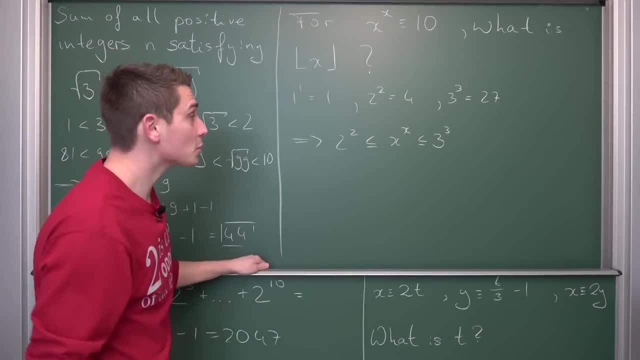 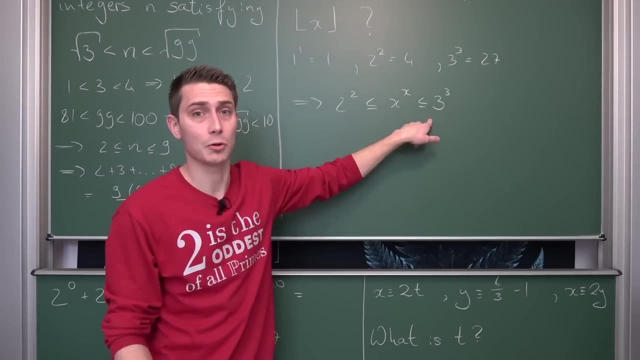 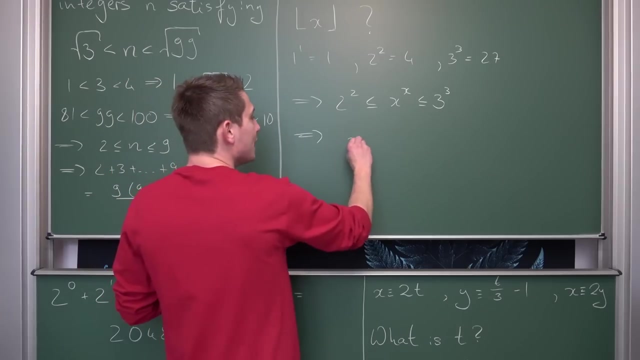 overall meaning. overall, you could make use of the lambda w function, but this would not really help you here in this case, because x to the x power on those bounds is only going to yield real solutions. now you can basically just compare bases and exponents. so this is giving us overall with 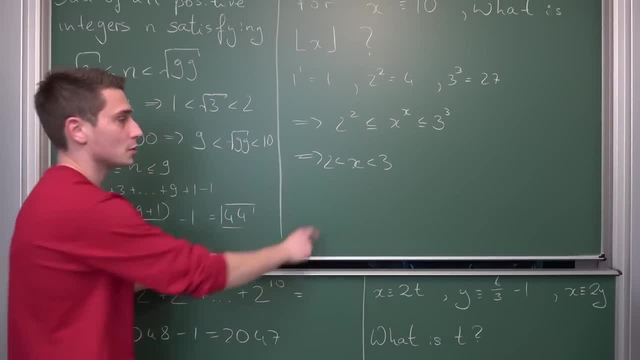 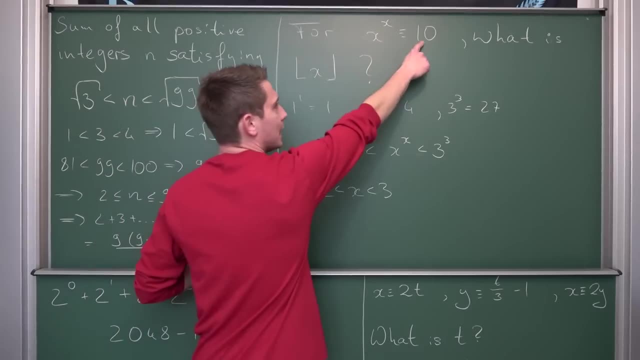 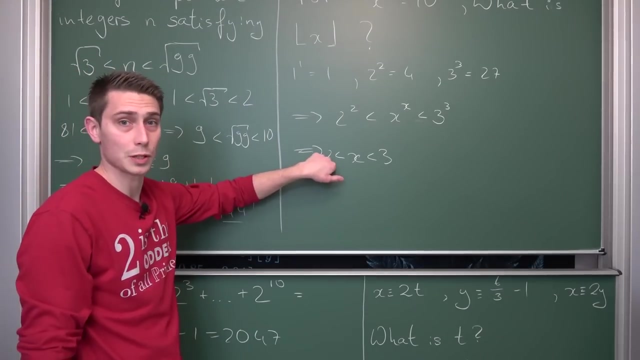 x being bounded between 2 and 3 and strictly between 2 and 3. I'm terribly sorry you can't have it equal to obviously, because x to the x power being equal to 10 implies that those can't be equal to. now if we have x being bounded between 2 and 3. 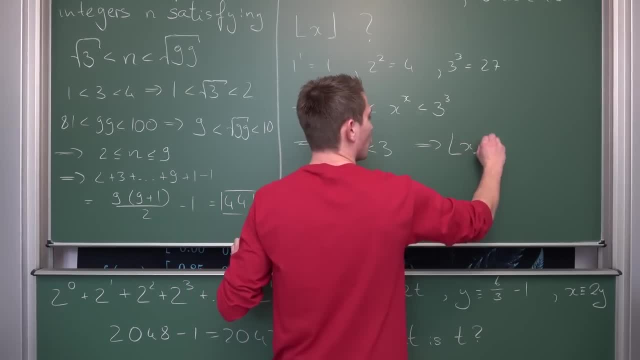 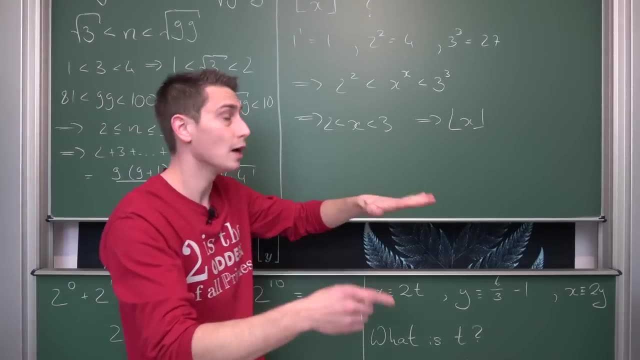 what happens if we take the floor of x? I mean, obviously, if we take the floor of x. x can be something from 2.000000000, blah, blah, blah, 1, let's say up until 2.9999999999, ok, something of that sort. 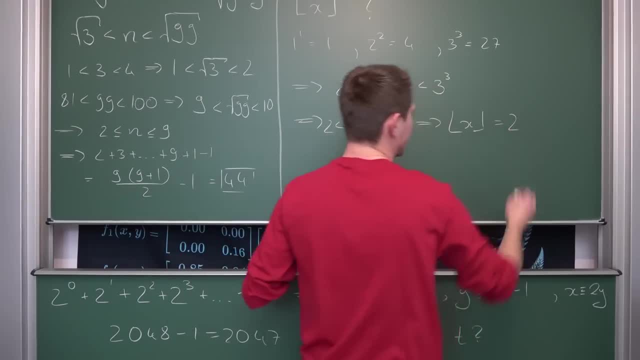 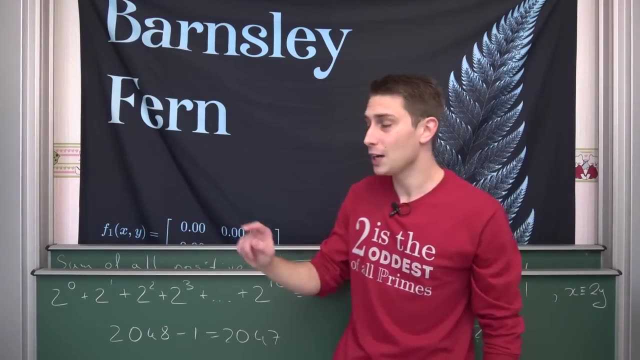 meaning if we were to round down our x, it's going to result in 2 overall. and this basically also concludes the last problem, and I hope you were able to figure everything out. if you are interested in seeing way more algebra calculus whatsoever problems, then I encourage you. 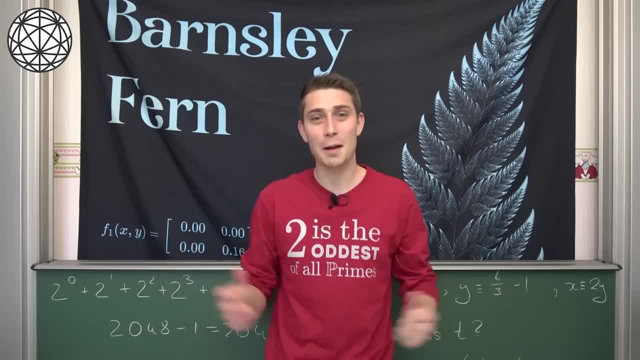 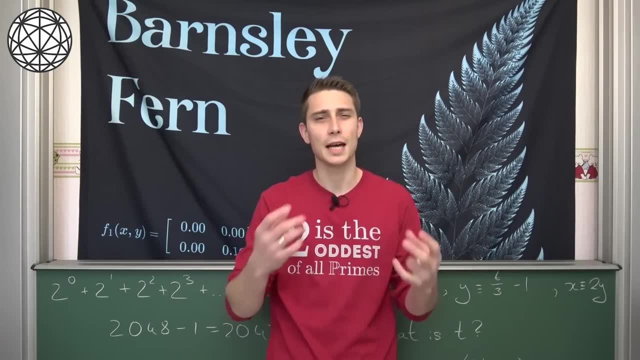 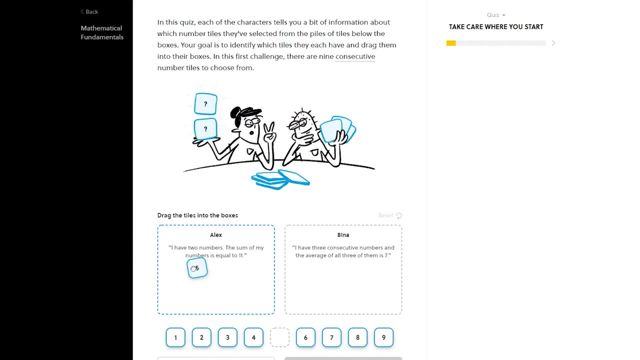 to try out today's sponsor, brilliant, who were kind enough to sponsor the last episode here of papa flammys advent calendar in last time. I take a lot of inspiration from brilliant because they just are able to provide a whole stem community with such a variety of problems and I really appreciate that. 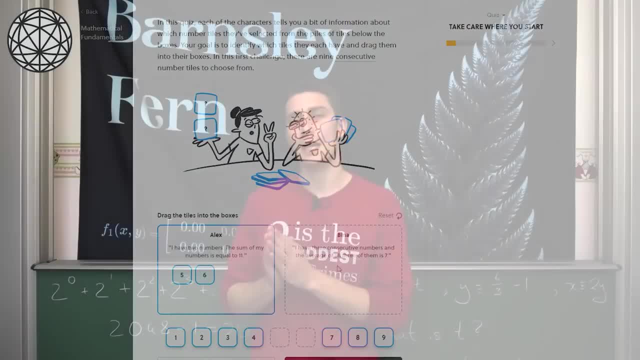 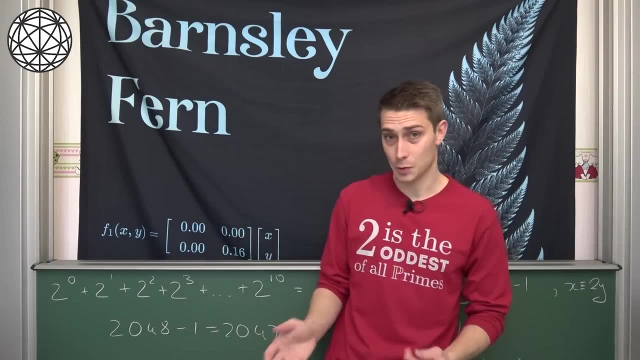 even from this advent calendar, 2 to 3 videos were actually problems that I found on brilliant and they were such a bliss to work through. sometimes they were easy, just like the problems we did today, but sometimes they were also kind of hard and took a lot of effort out of me to actually 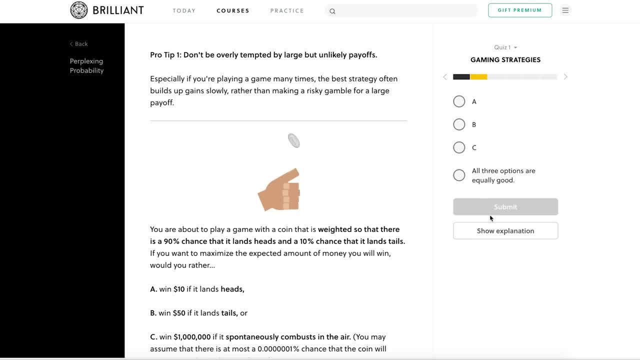 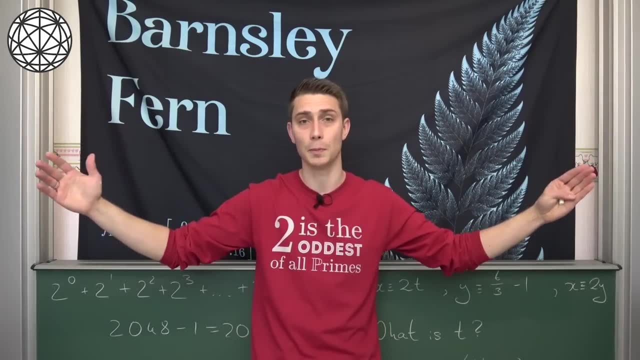 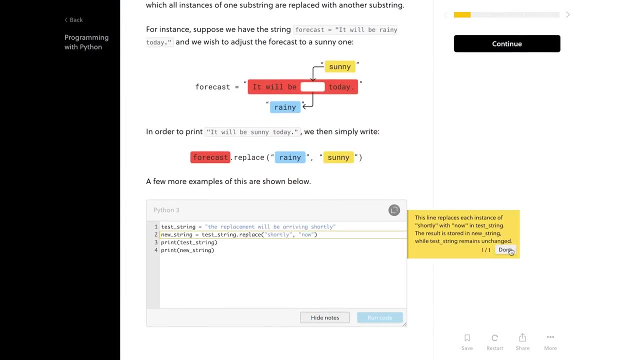 figure out, and this is what I appreciate of brilliant the most. they provide their whole community with a wide variety and range. of difficulties in problems often stem, be it physics, chemistry, mathematics, computer science, problems in topics. they got all of them and even more than that. 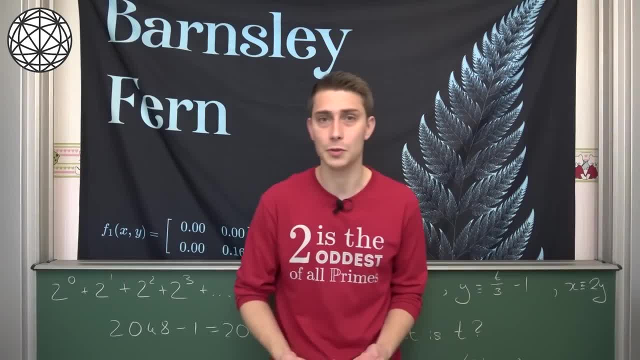 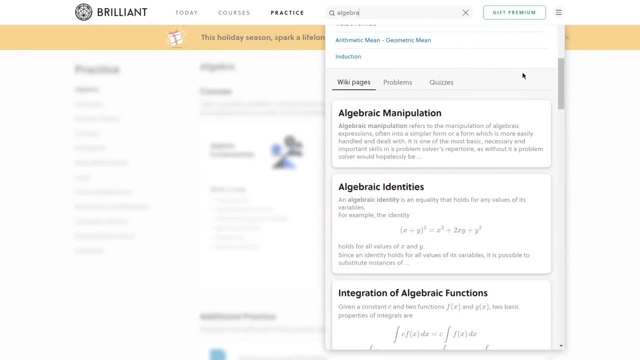 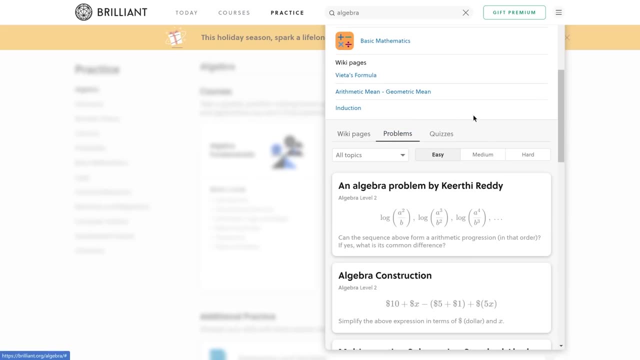 those problems, like mentioned before, came from the brilliant community, and the community is built out of brilliant members, obviously, which can contribute to their wikipedia pages and also their community and challenge pages, and I think it's such a great community because they also have to provide all the users with their 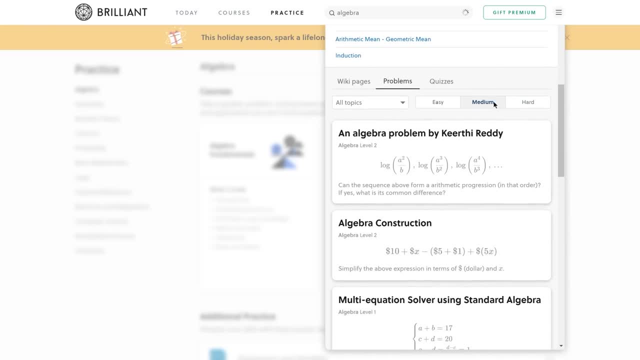 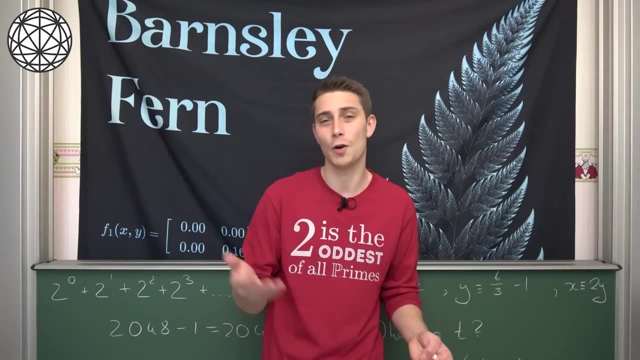 detailed solutions, and I think this is something that everyone really benefits from. even if you have doubts about your own solutions, you can just check what the community did and you can also vote if the answer was helpful or not so helpful, etc. so this is something that I really appreciate. 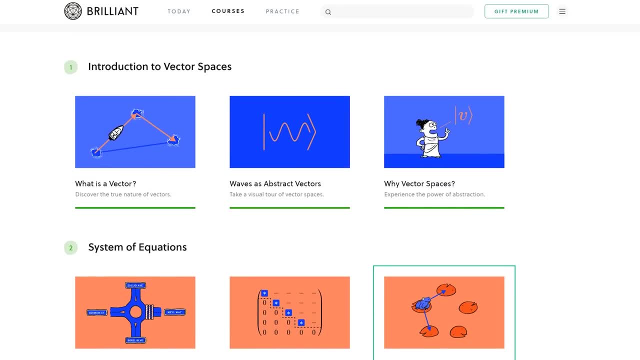 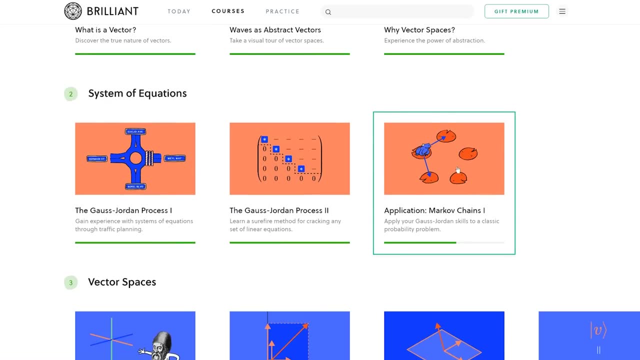 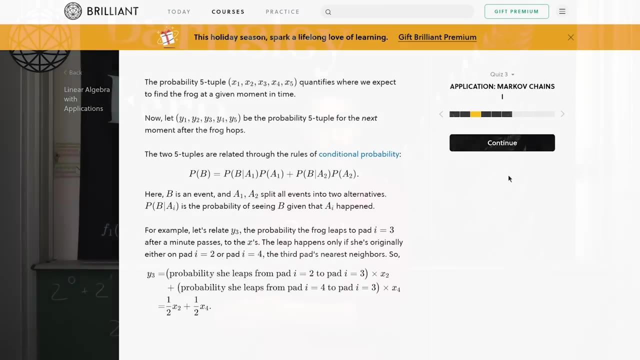 just like with brilliant's course concept, starting up from easy problems, they are going to get harder and harder gradually, giving you an overview of all the most important topics you are going to need, starting from high school life up until university life. even on brilliant, I heard for the first time of markov chains. 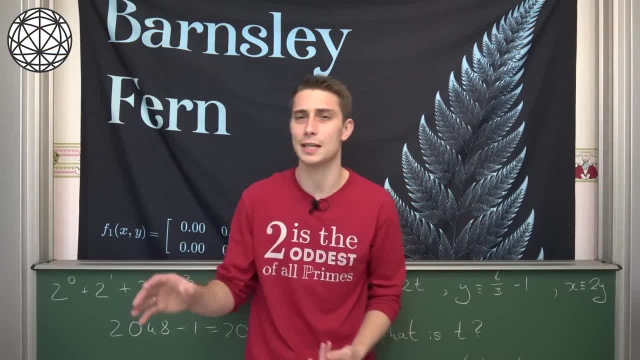 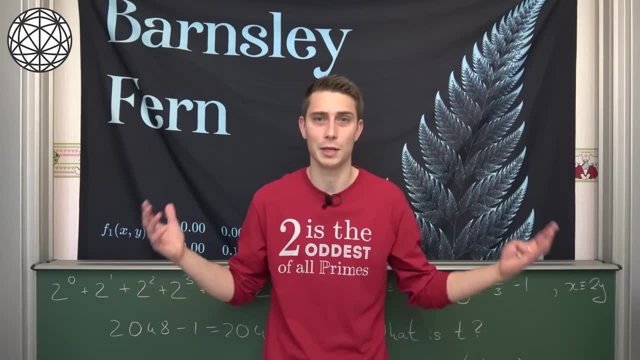 for example. I mean, I scratched the surface at university already, but I never got into too much detail about markov chains, and this is something that, for example, brilliant offered to me, which I find highly pleasing. so if you also wanna try out brilliant, if you wanna support the channel, 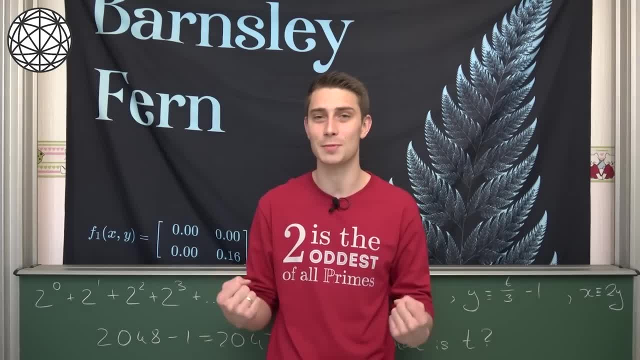 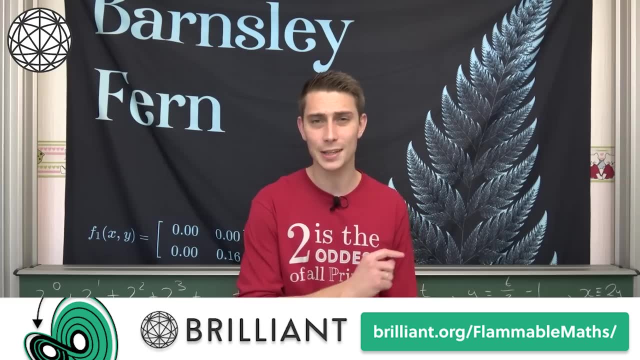 if you think that this could make for a very nice last minute christmas present, then make sure to check out the link at the top of the description. with it, you are going to get 20% of an annual premium subscription if you really use it, but other than that you can. 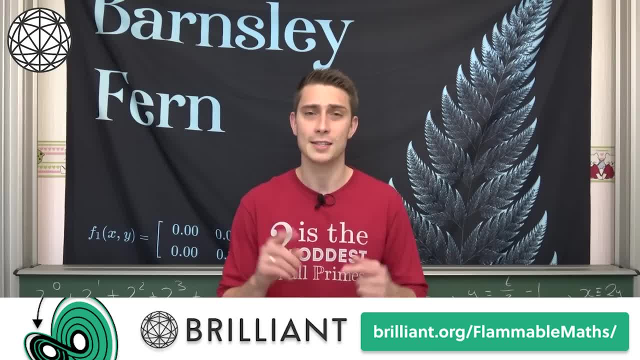 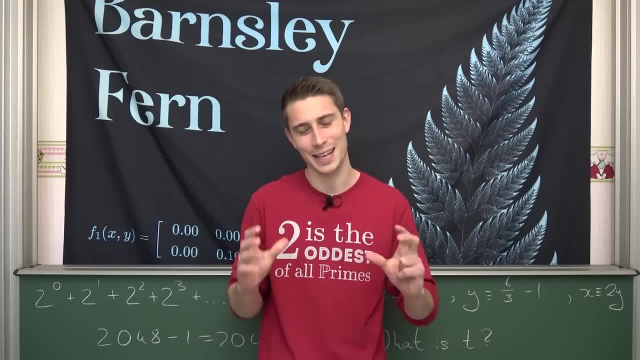 just click on it and try out a big portion of brilliant already for free. so that's a really great deal considering how much content they already have on their website, and it's such a lot of fun to work through their problems and all the animations and interactive. 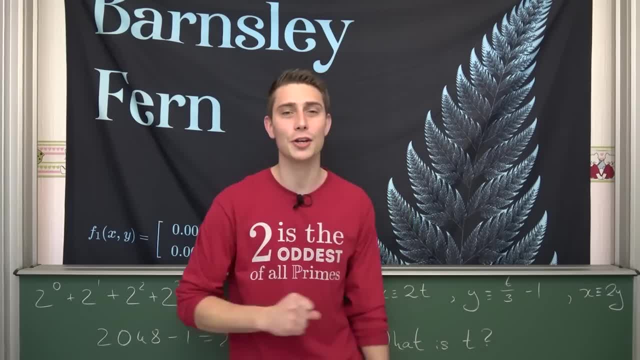 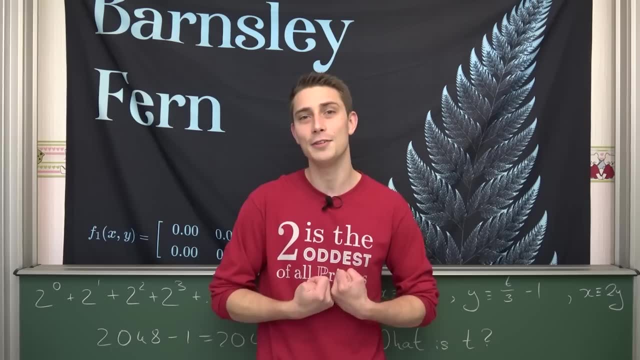 and interactive problems are just really nice to work through. so, yeah, give it a shot and support the channel this way. if you enjoyed this video, please subscribe and recommend the channel if you like- and I hope you did enjoy- pop up lemmy's advent calendar, and if you did, then definitely.